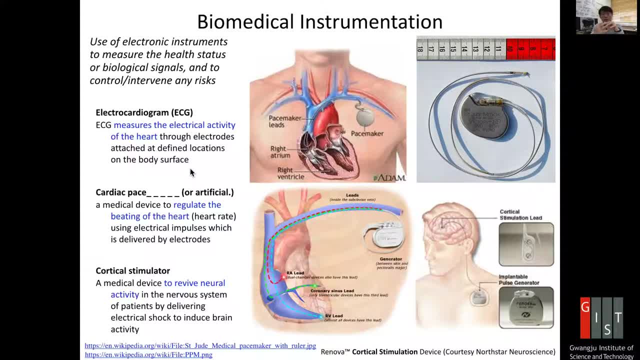 And those patients may have irregular heartbeat which may cause increase of risk And we can have an intervention to externally sending signal to the heart to contract at a regular fashion And that is called pacemaking. So here is called cardiac pacemaker. 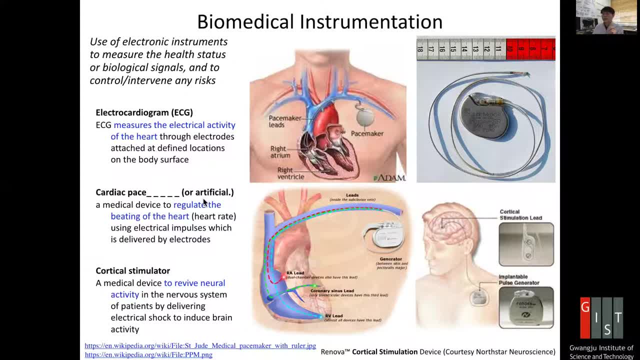 Or we call it artificial pacemaker. This is a medical device to regulate the beating of the heart. Of course, heart rate can be regulated by using sending electrical impulses, which is delivered directly through electrodes inside heart muscle, And another example is called cortical stimulator. 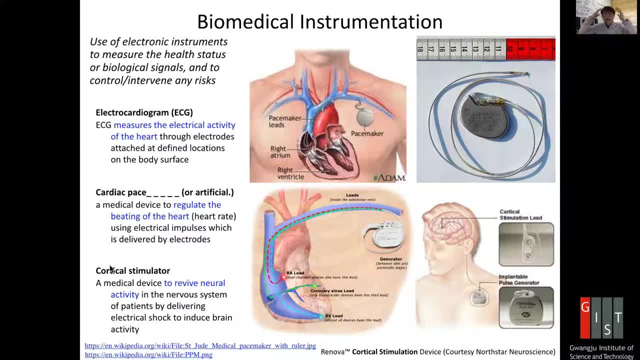 And this cortex means in fact the outer layer of the brain, So cerebral cortex. So this medical device is to revive neural activity in the nervous system of patients by delivering electrical shock to induce brain activity. So let's take a look for this cardiac pacemaker, which is about this small size. 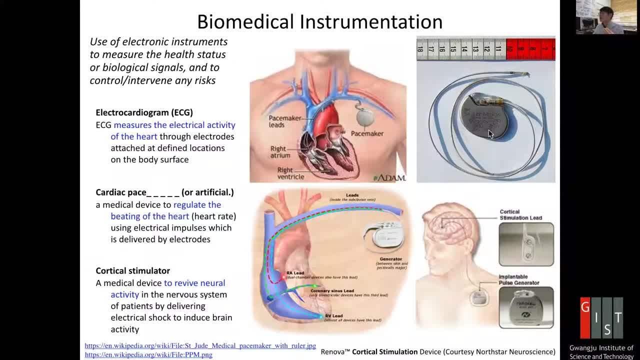 It's not very big And this contains a big plate. It's a battery which sends out electrical impulses through this electrode And if you look at this it's a little bit tiny. But at the tip of the electrode it is a wire which is whoring and neater, so that you actually insert into the heart by rotating and then fix it. 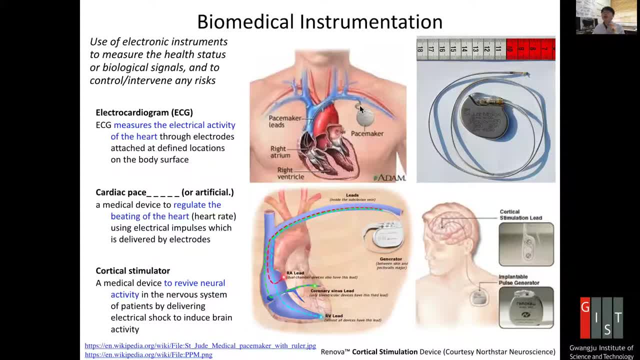 So this pacemaker lead goes through the wall of the vein And the vein which is connected directly to the heart, from your heart anatomy knowledge, these veins goes to right atrium And its right atrium is connected to right ventricle. 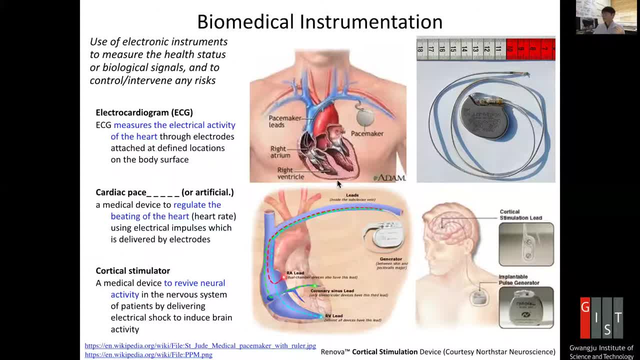 So it goes to tip of the right ventricle. So, more specifically, you can see, So this generator is placed surgically inside the body And it goes to subclavian vein Which is connected to right atrium And you can have right atrial lead or coronary sinus lead or right ventricle lead. 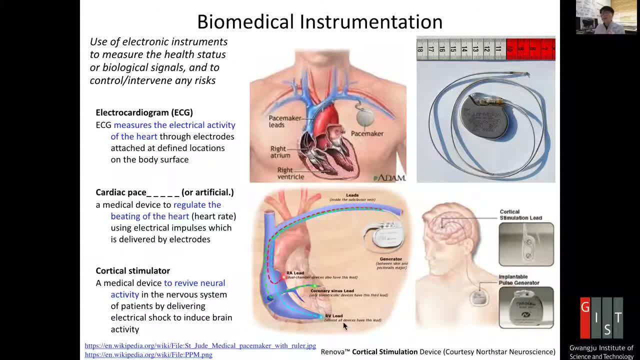 And this right ventricle lead is. almost all device has this lead And the cortical stimulator, which specifically placed in the brain cortex. So cortical stimulator lead looks like this And that also is connected to the body called implantable pulse generator. 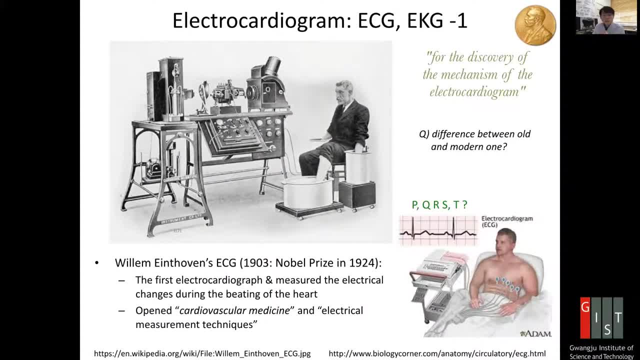 Then who actually first measured this heart electrical activity? So that heart is electrical device And that electrical activity can be measured, So humans invented electro, and cardio means heart And gram means graft, So heart activities, electrical property can be made visible. So that Wilhelm Eindhoven first created this in 1903. 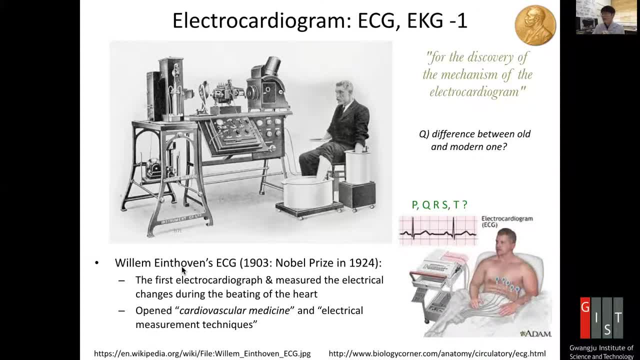 He's Dutch and he's a doctor, And he was the one who first create this device To measure the electrical activity, To measure the electrical changes during the beating of the heart, And so he's the father of cardiovascular medicine. And by electrical measurement techniques. 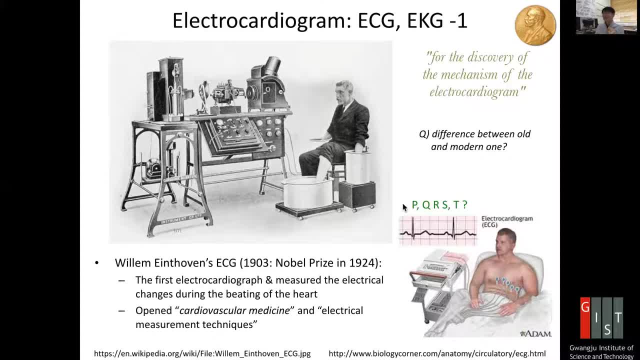 So for this discovery of mechanism of electrocardiogram He got awarded Nobel Prize in 1924.. And look at this How big the machine is. And what's interesting here Is he merged his two arms, This back and one back. 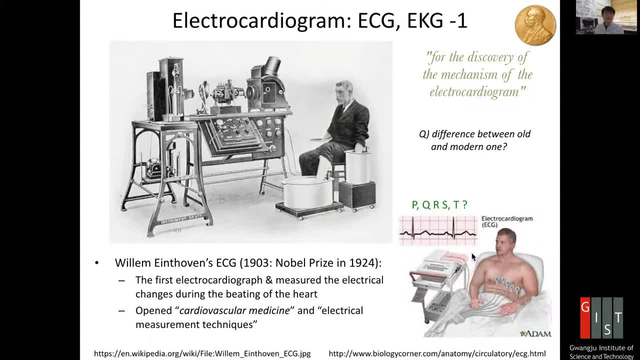 Compare this size with a modern ECG machine Which, when we go to the hospital for regular checkup, The nurse put this attached electrode on our chest And we also have electrodes onto our limbs, Two arms and legs, And that small tiny machine will show up this ECG activity. 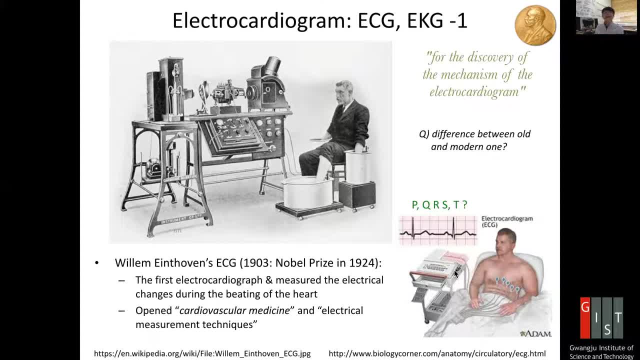 So what's the difference between old and modern one? I would say, in principle it doesn't change much. And these electrocardiogram, The shape, not that different, And people named it as a P, QRS, T, Something like this pattern: 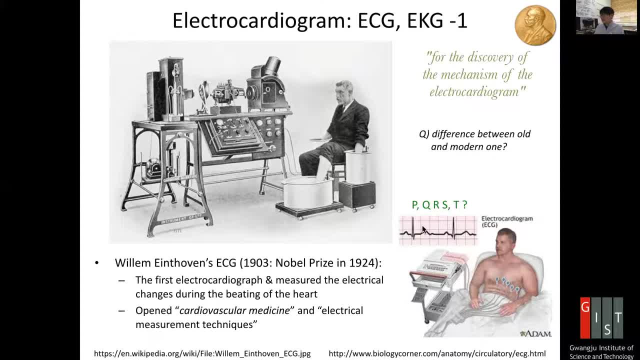 People named it. So the difference between these are, You see, the size. And in the past People put a salt water bag So to immerse, Because this is electrically conductable water And while nowadays we can just attach electrodes. 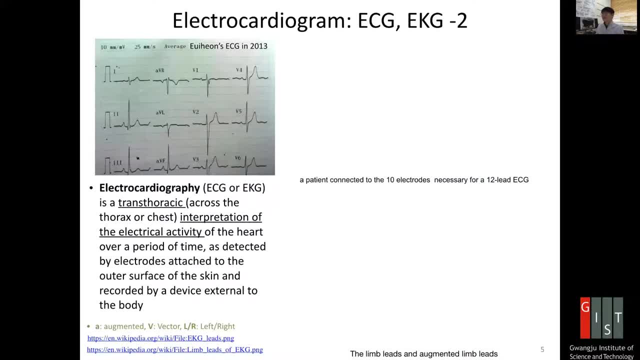 A simple way. So I brought my own ECG diagram, Which I bagged for the nurse. Please give me this So that I can share with my students. So look at this. This is recorded in 2013.. I've got this strip of my ECG diagram. 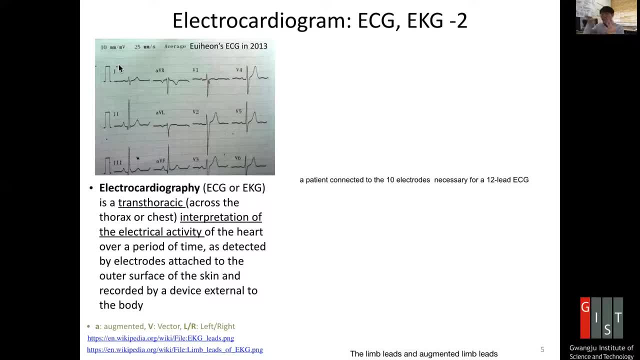 Which is written on top of this grid line: Just one millimeter, And this grid line has a meaning. So, for example, in vertical Amplitude aspects, 10 millimeter of grid line Means one millivolt, Okay. And the x-axis is: 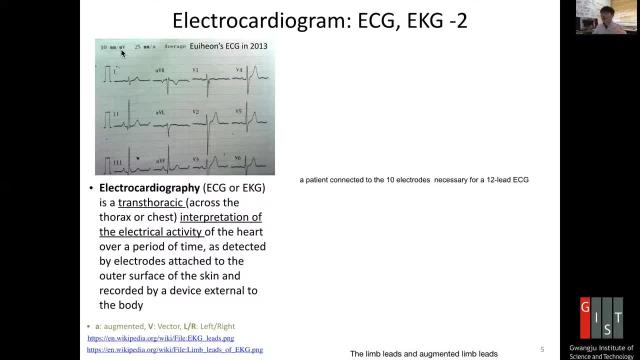 While the heart is beating. So the speed of recording Is 25 millimeter Corresponds to one second. So that you know exactly The speed And temporal domain And this amplitude, The strength of the electrical activity. And one thing you notice is here: 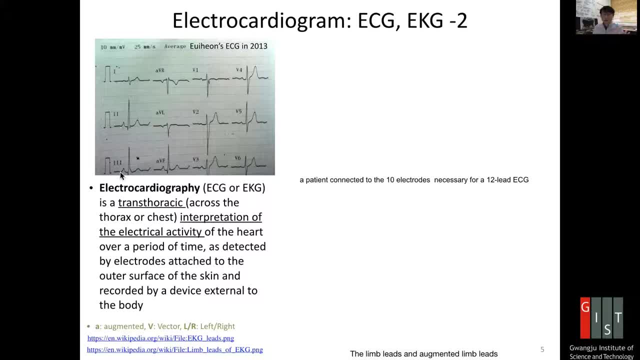 I Double, I Triple, I And V123456.. And there's AVR, AVL And AVA, F, So total about 12.. Lead ECG Can be displayed here, And this Is in fact Our heart activity. 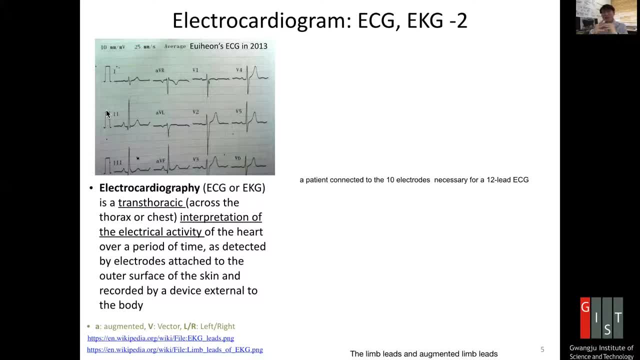 So one Rhythmic activity Is, as I said, It's a three dimensional Dynamic activity, So the Net vector Of electric Vector Can be actually changing in 3D, So For us And physicians To be able to see. 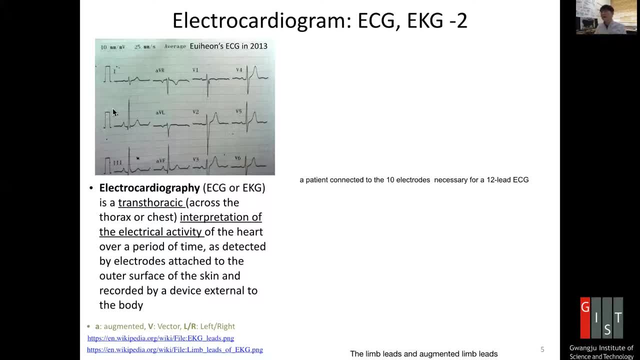 This easily. We decompose This Into This 12. Aspects. So, Like When I was taking this, This is me And you see One, Two, Three, Four, Five, Six. Lead is on my chest. 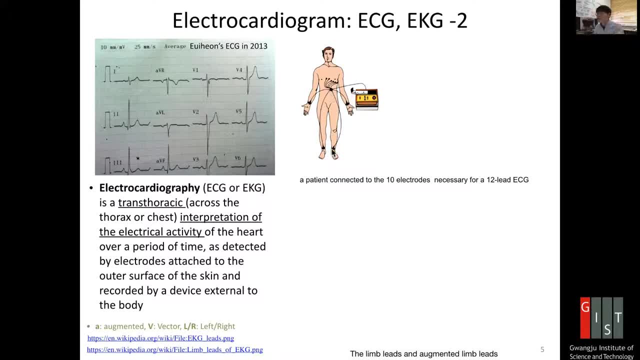 While I wasn't naked. Here, Two Leads Onto my arm And Two Leads Onto my foot. So The, The, The geometry. So This V1. To V6. Is showing 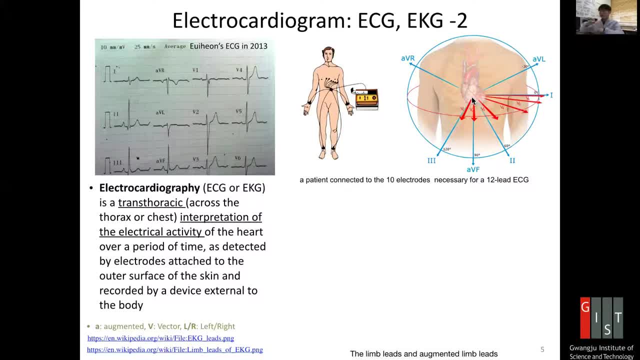 The electrical vector Onto This Plane Cut across A plane While There's a This Plane. My In Plane Is I, Double, I, Triple I, And also Vector Right. 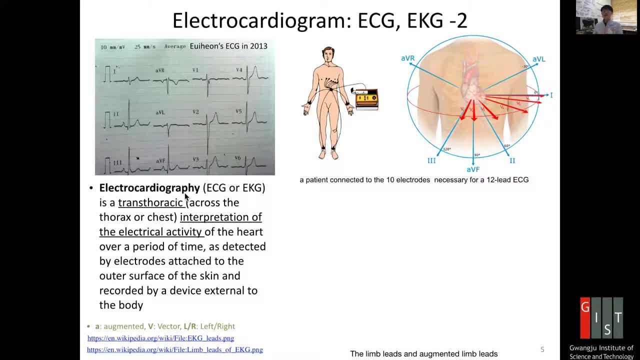 And Augmented Vector Foot. So This Electrocardiography ECG Or In German Term EKG, Is A Trans Thoracic Meaning That Across Thorax Or 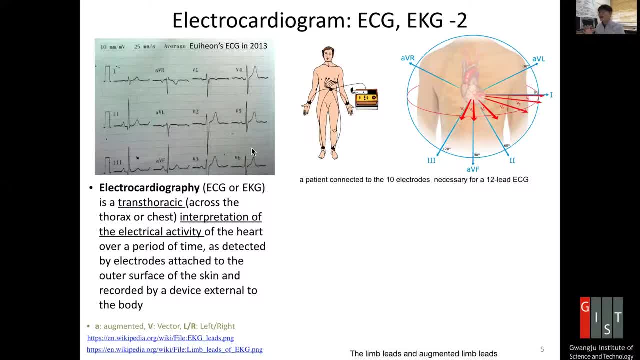 Chest: Interpretation Of Electrical Activity Of The Body. So How Do We Want To Visualize This Three Dimension Electrical Vector By Having This Twelve Electric? 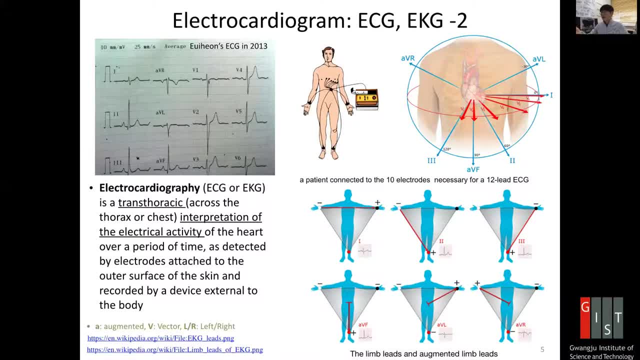 Electro The Lead. So Very Simple Way, We Have This Two Arm And Foot As A Inverse Triangle. So From Vector Point Of View, You 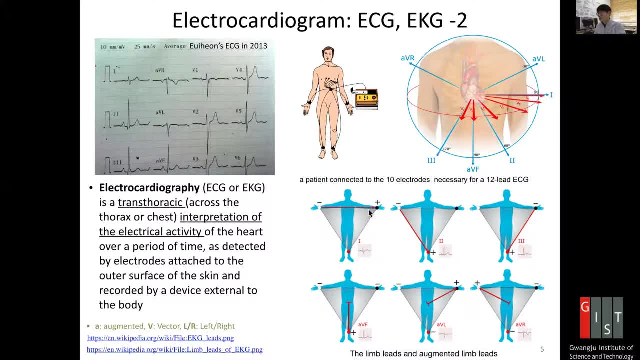 Can Make An Easy Way. So Let's Say, Subtract From Left Arm To Right Arm, Then We Can Create This Vector And Likewise Foot Subtracted. 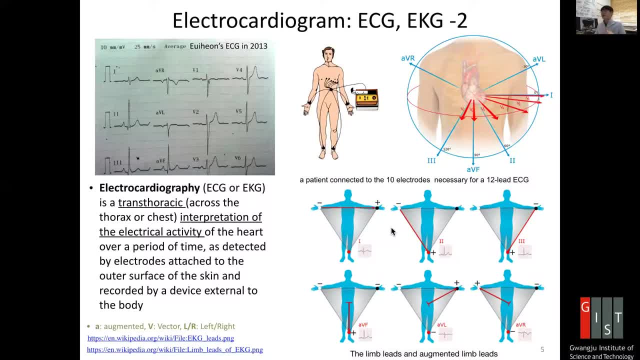 Foot By Left Arm, Create This Vector. So This Create Three Ways Of Vector In Plane. So This Is Consider The Body As Like Three. This 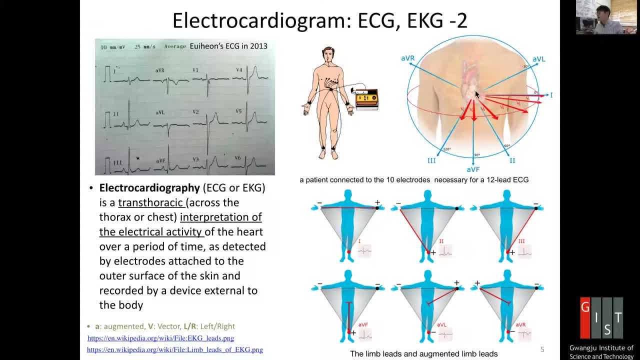 Hundred Sixty Degree As A Part, As A hundred Twenty Degrees. So This AVL, AVR, AVF Was. You Can Create This. This Is Vector Downwards. 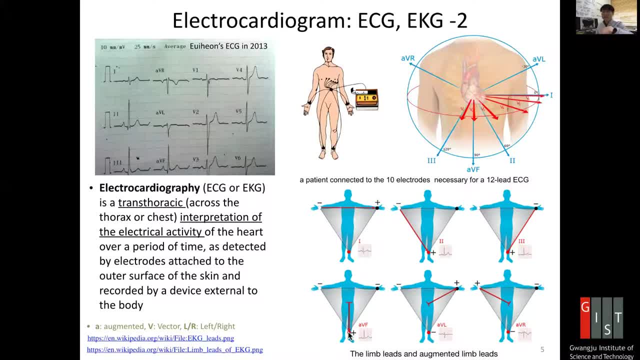 To The Foot Side, So It's Called Augmented Vector To The Foot. Likewise, From From This Average. From This Average, You Can Subtract From The. 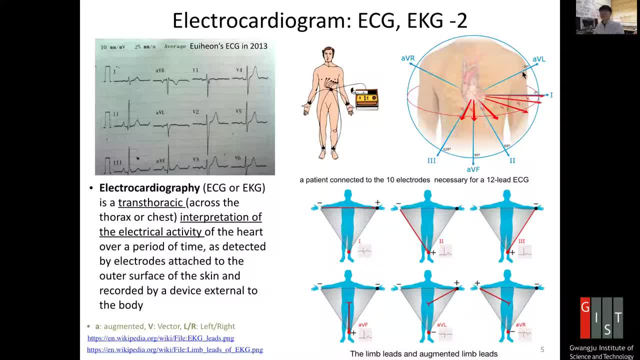 Left Arm Towards Foot. Augmented Vector: Towards Left Arm, Towards Right Arm. As You See, Minus Thirty Degree, Sixty Degree, Ninety Degree, Hundred Twenty. 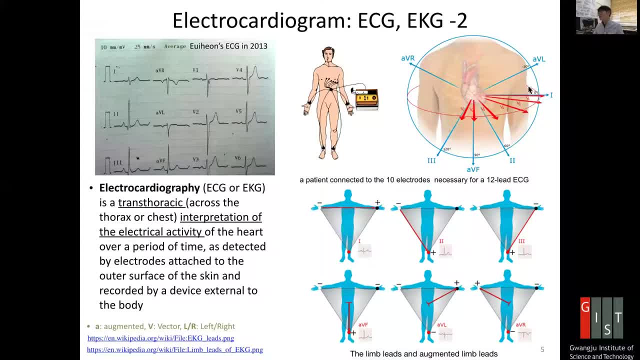 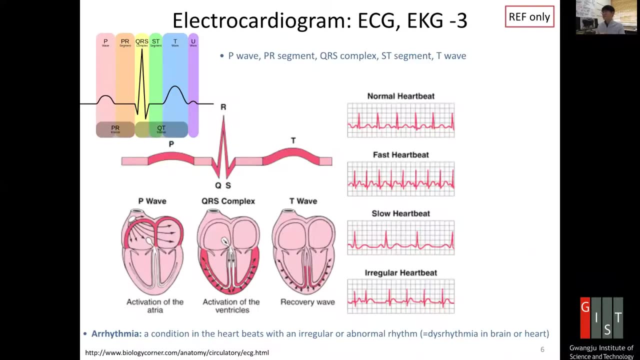 Degree. So This Way In Plane Activity Of The Heart Beat And The Heart Is There, Like The Entity Is There, And These Are The Projection. 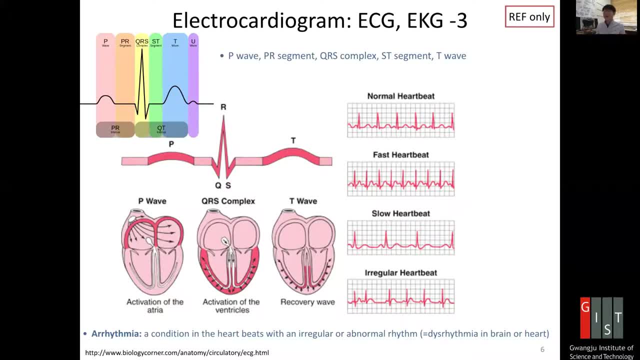 For Easy Interpretation Of Physicians. So So What Does This Electrocardiogram Mean? That The Atrium, Which Is A Smaller Room With A 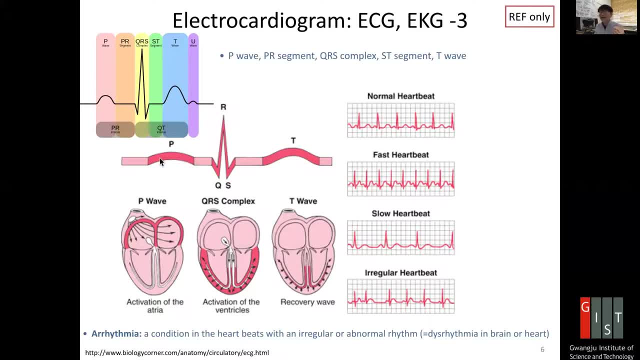 Floppy Muscles And Which Can. This Contraction Of The Atrium Causes An Electrical Activity, Here A Little Bit Small, Which Is Most Powerful. 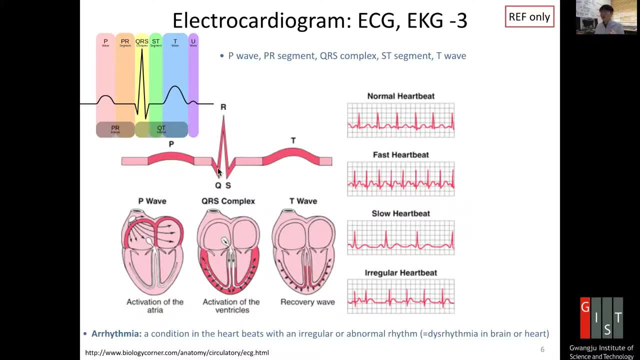 Real Pumping Action, So That Is At Highest Amplitude, And We We Call This As A Q R S Complex, And Then It Has To. 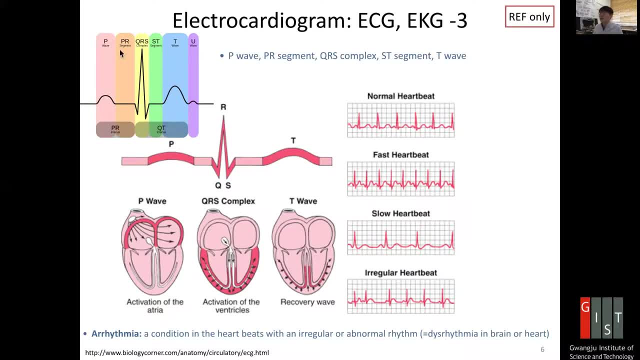 Recover The Positioning Of Your Heart. So This P As A Wave And Q R As A Complex, And T As A Wave. We Also 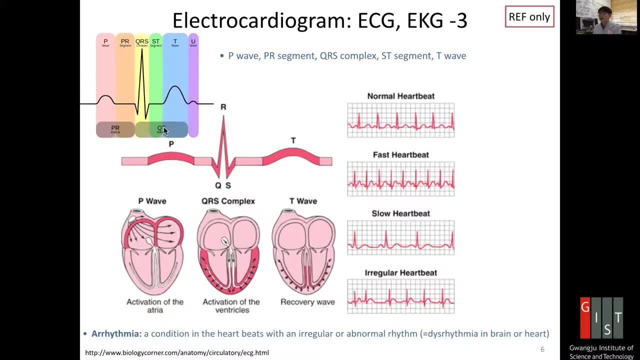 Are Interested In The Interval Of Your Heart ECG. So The Normal Heart Beat Looks Like This And We Know Normal Heart Beat Is Usually. 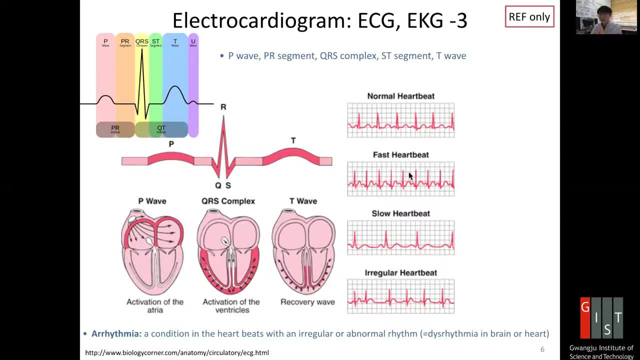 From 60. To 100. Beats Per Minute. If It's Slow Heart Beat, Of Course. If It's Irregular, That Is Call, Become A Problem. 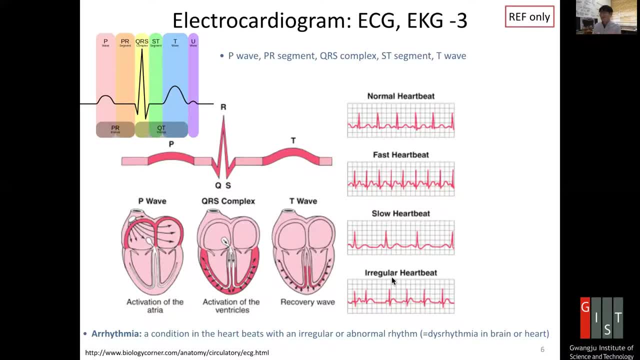 And That Be Called Irregular Heart Beat. But Physicians User Uses Jargon Which Is More Complicated: Fast And Slow Heart Beat. They Call Bradycardia. 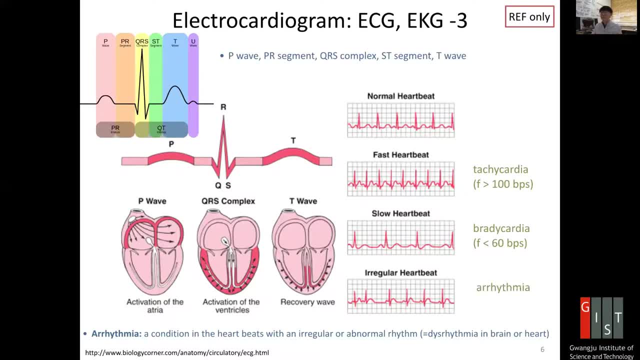 Brady Means Slow. An Irregular Heart Beat Is A Serious Condition That We Call It Arrhythmia. So Arrhythmia Is A Condition To Function. 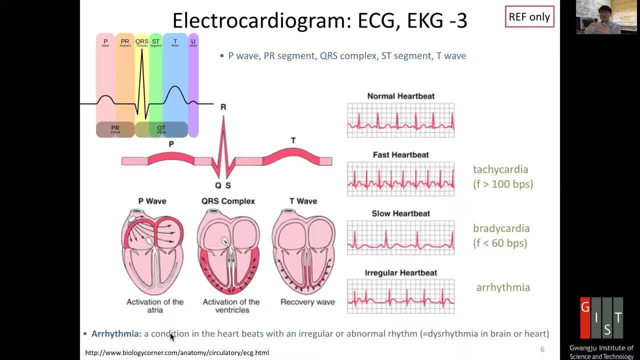 As A Pump To Send Out Oxygenated Blood Throughout To The Body And Then Collect Those Deoxygenated Blood To The Heart. It Has To. 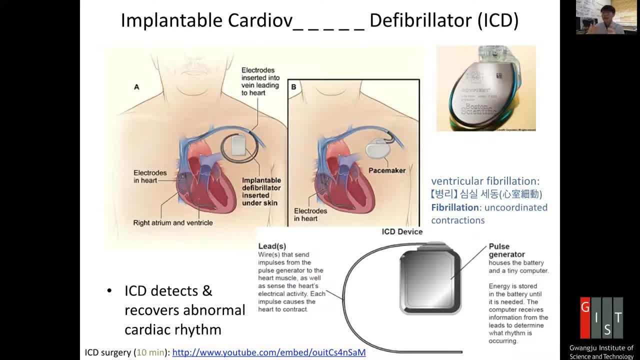 Be Coordinated, So This Arrhythmia Condition Have A Tendency To Enter Into A Real Uncoordinated Contraction, Which Means You Know The Ventricle. 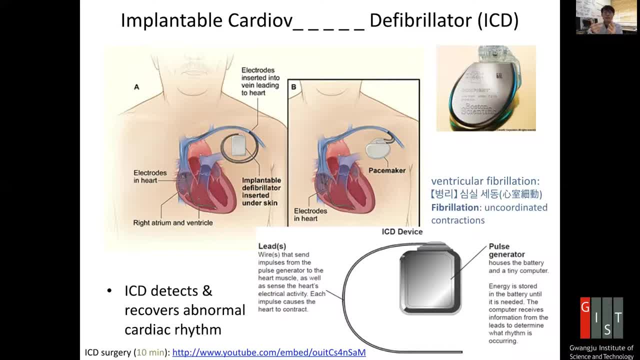 Has To, Has To Pump In This Way. But If This Phenomena Is Happening, Then We Have To Give Electrical Shock To Recover, Like 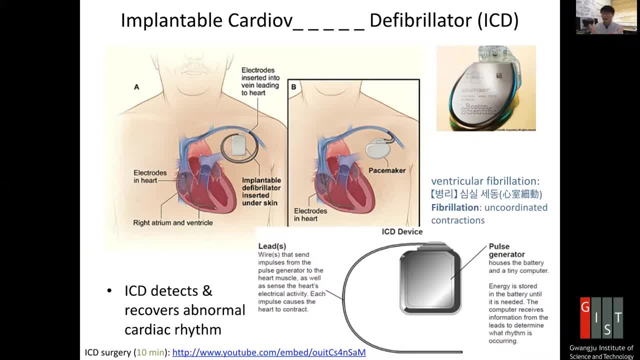 Reset The Heart So That It Can Recover Its Normal Rhythm. So This Can Save A Uncoordinated Contraction. So This Is A Very Serious 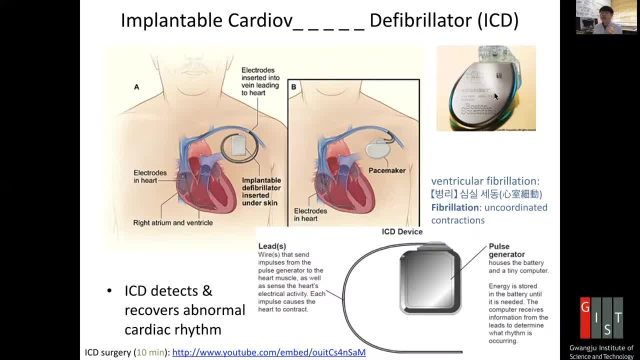 Condition And For That Biomedical Engineer Device, This Implement Implantable Device Which Will Defibrillate This, So Meaning, You Know, Recover From Implantable. 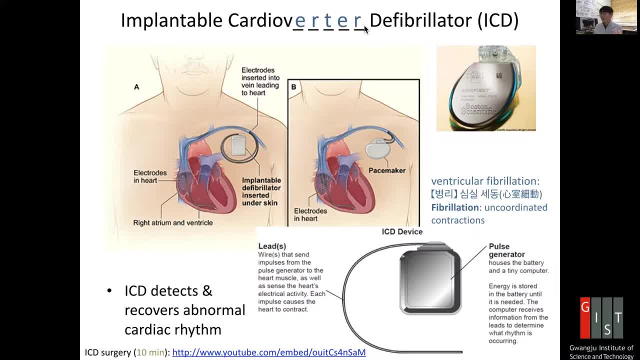 Cardio Vector Defibrillator. And What's The Difference Between The Pacemaker And This ICD? It Looks Quite Similar Upfront, But Pacemaker The Goal. 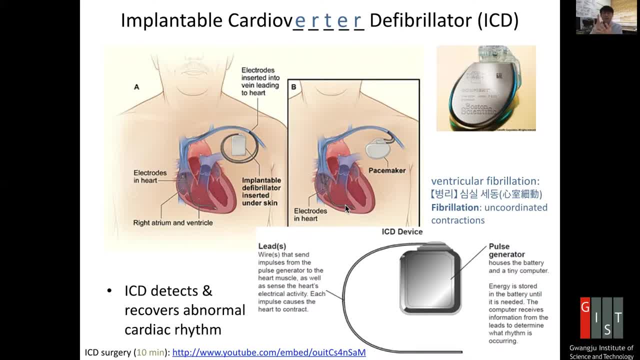 Of This Pacemaker Is To Make The Vector Defibrillator Has To Listen To The Heart ECG In Real Time, So That It Has To 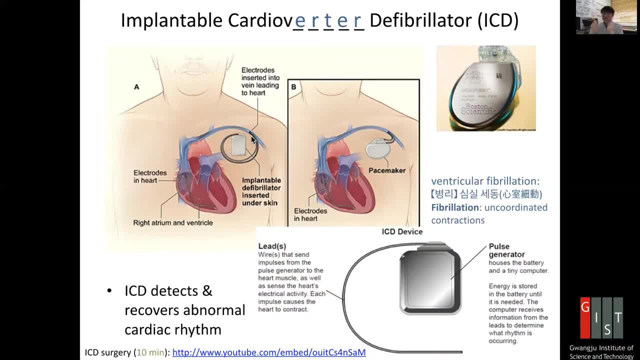 Read The Heart Signal ECG And It Has To Have An. So This Implantable Cardio Vector Defibrillator Actually Has To Detect And Recovered. 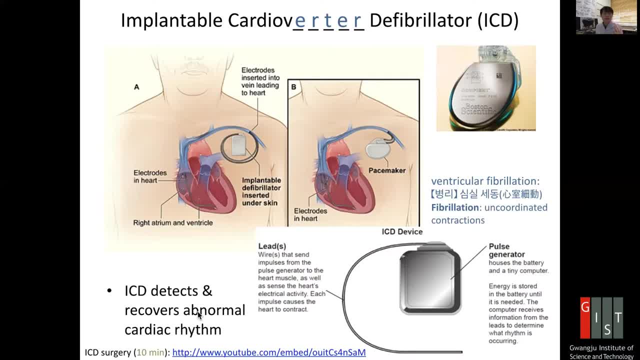 Abnormal Cardio Rhythm. So To Insert, Implant This Device. Patient Has Needs A Surgery And I Found This Medical Process. Look Like What Kind.